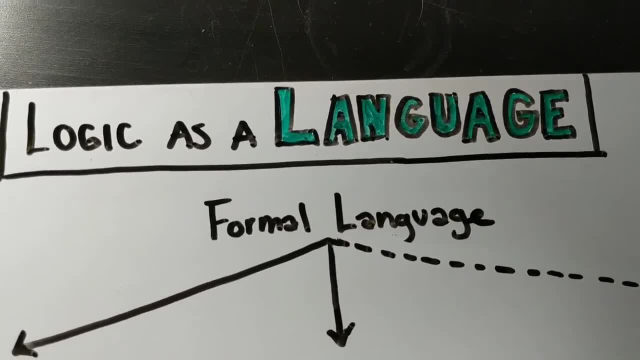 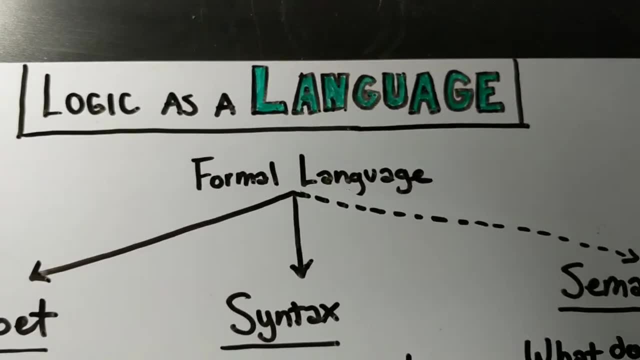 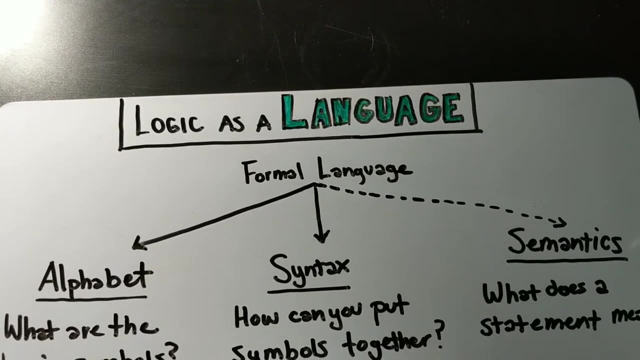 formally as as something that we're breaking down into in modeling. formally, A formal language typically comes with three sets of information. It comes with an attitude, structure, alphabet, a syntax and usually a semantics. So that's not actually required. You can have a. 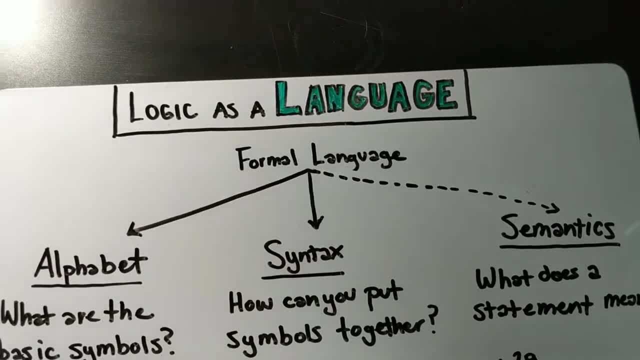 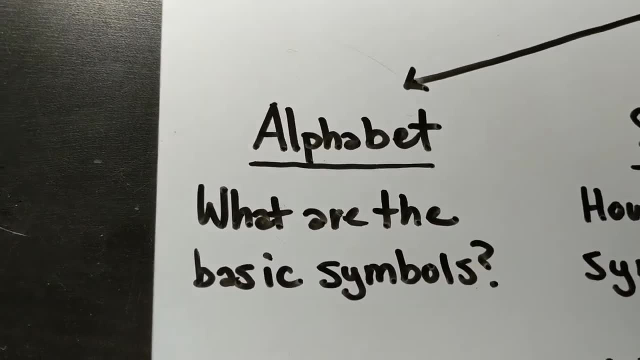 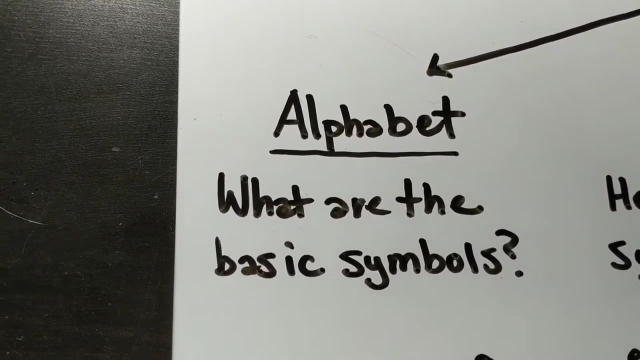 formal language that has no meaning. It's just a series of meaningless things, So we'll talk about each of these in turn. So an alphabet. what we mean by an alphabet is that a formal language has to have a set of basic symbols. right? These symbols could be anything from little. 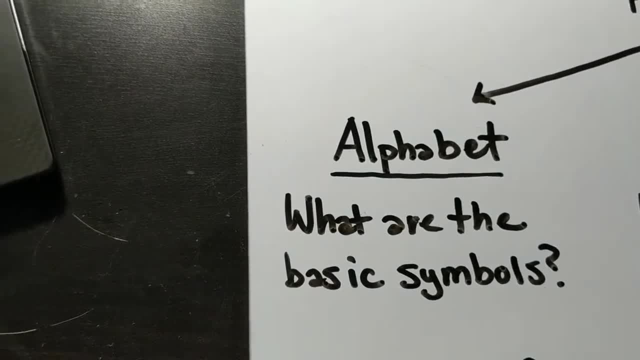 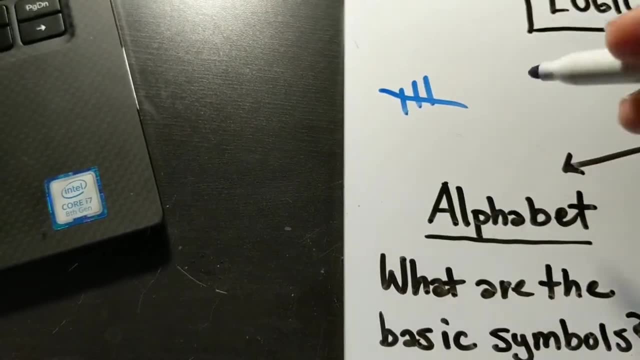 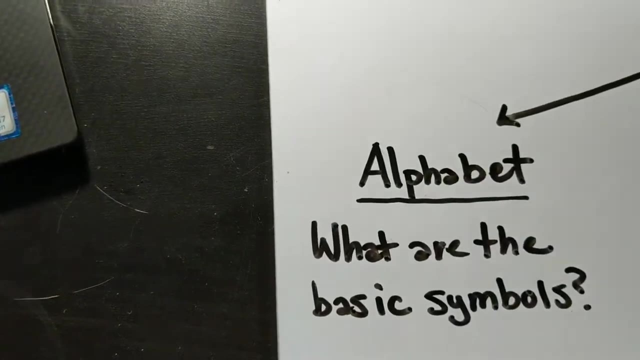 you know doohickeys on a page, which could be something like you know tick marks and cross ticks, for example, could be your symbols, right, Or it could be something as complicated as whole words, for example, could be your alphabet. So what we mean by an alphabet? 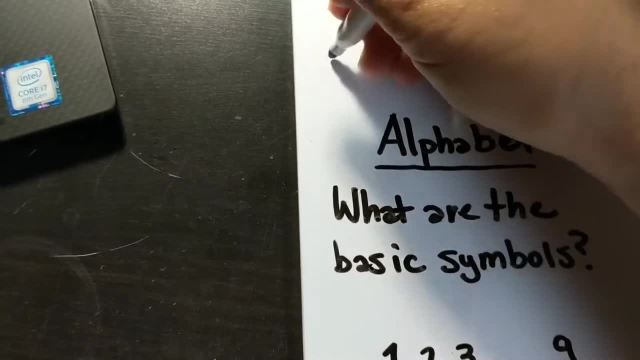 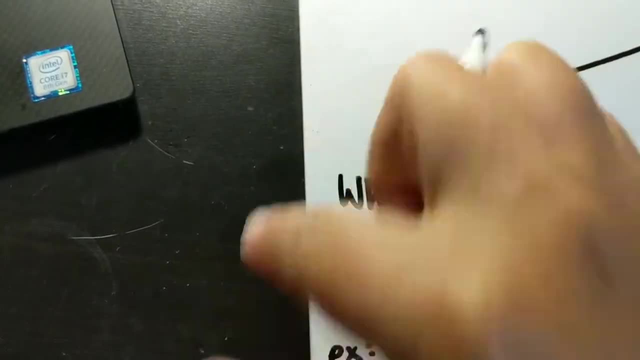 the word alphabet is sometimes confusing because it conjures you know A B C in your mind, but alphabet includes a lot more than just A B C, Or maybe even a lot less than just A B C. It's just whatever your basic symbols are. 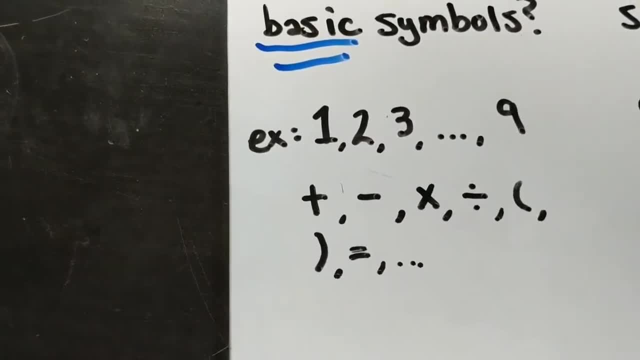 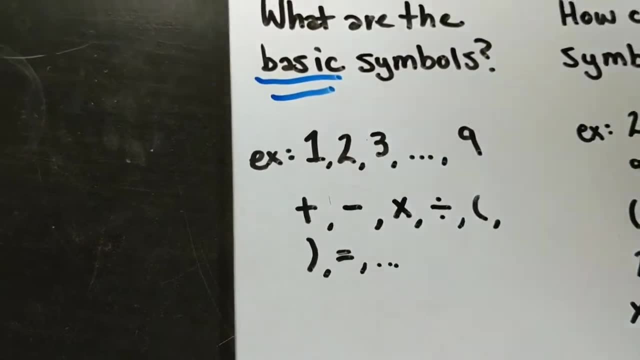 So, for example, you all are very familiar with the formal language of mathematics And some of the basic symbols of mathematics are given here. right, This is the alphabet right. We have a series of numerals right Which we can combine in different ways, right? But these? 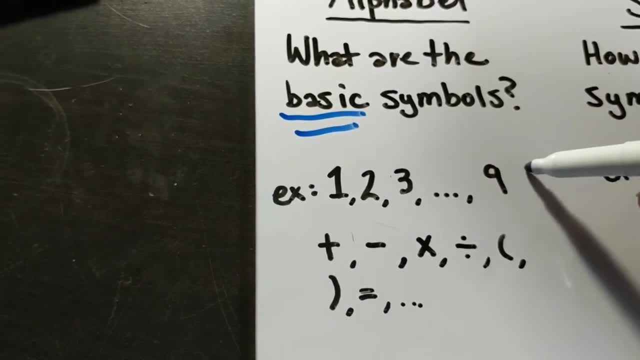 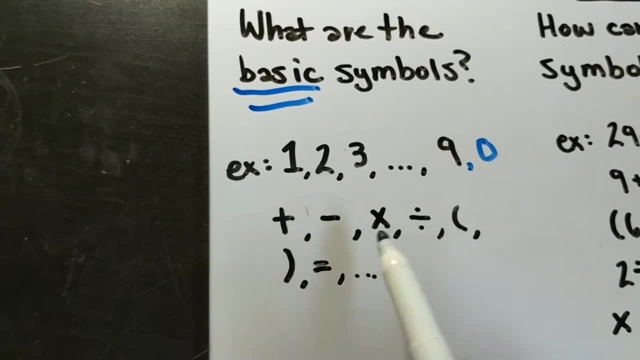 are the basic numerals. is the numerals? Oh, I guess we have to include zero too, right? These are the basic numerals of um of mathematics. But then you also have some operators. There's a lot more operators than. 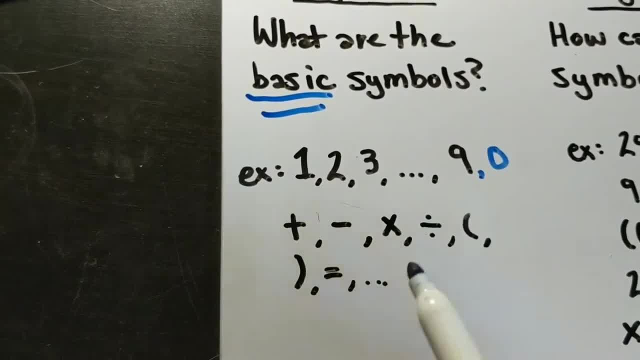 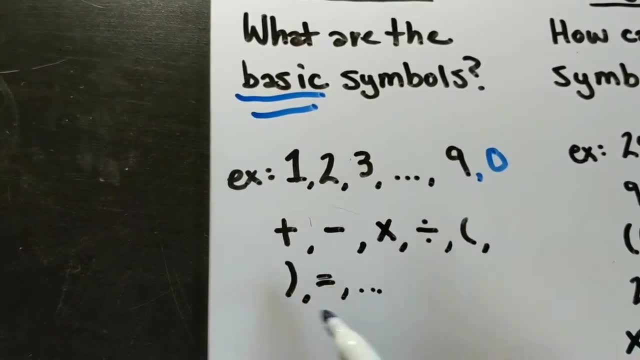 this, right, But these are the basic symbols that you see when you're doing math, right? And you can add a lot more to these lists, obviously right, But the basic symbols are your alphabet, the symbols that you're going to combine with each other. We've also recently been working on set. 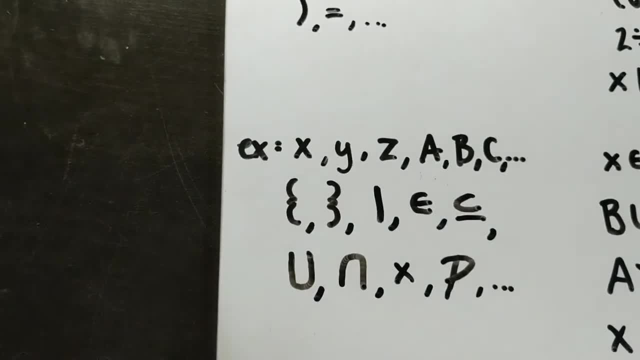 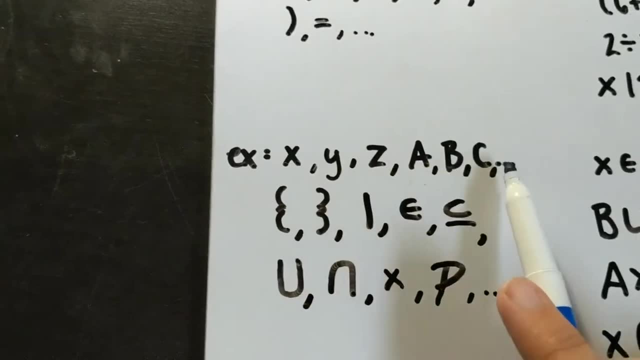 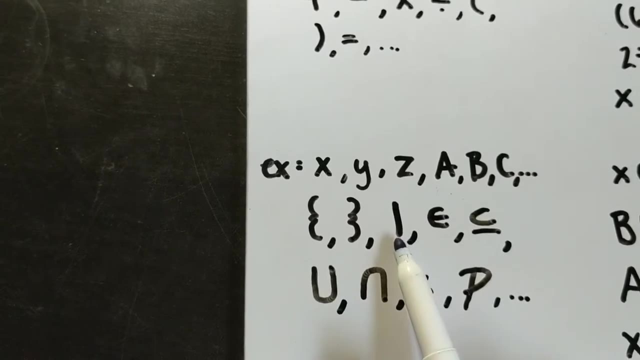 theory and this has a slightly different set of symbols from regular basic mathematics. right, We have lowercase letters. we have uppercase letters that denote sets, usually, but not always. Um. we have set brackets. we have this um which we use in set builder notation. we have this: 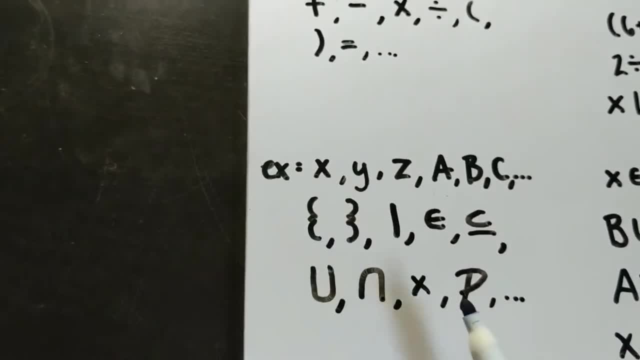 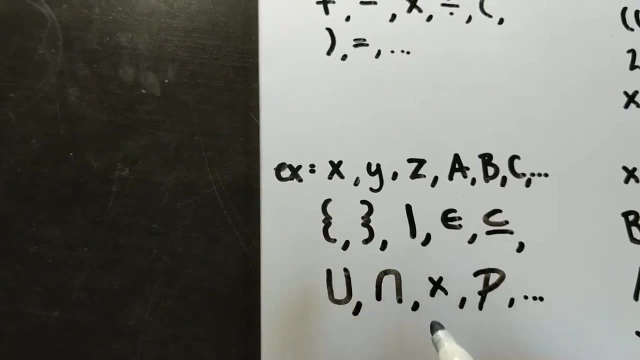 membership thing, right? So we have all these different symbols um, which we will combine in different ways, But these are the basic symbols that you can use, And so this is the alphabet of set theory. We will talk about the alphabet of formal logic as we go along as well. All right, so? 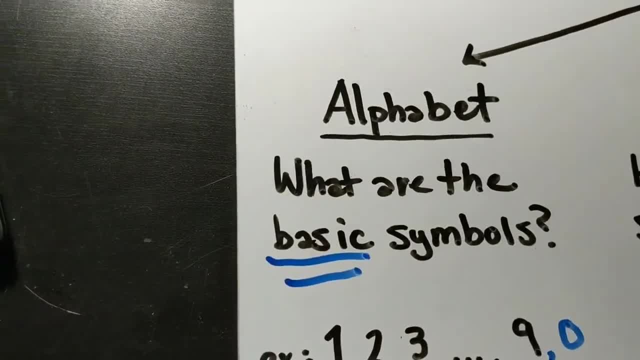 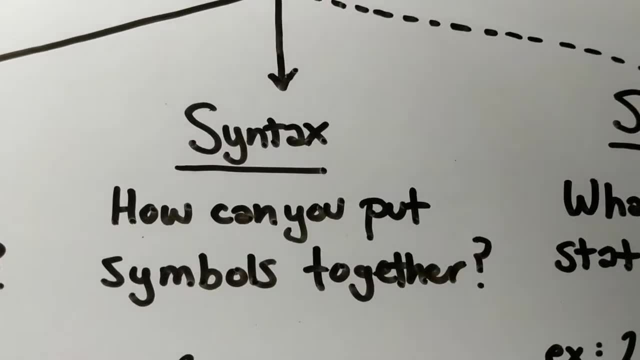 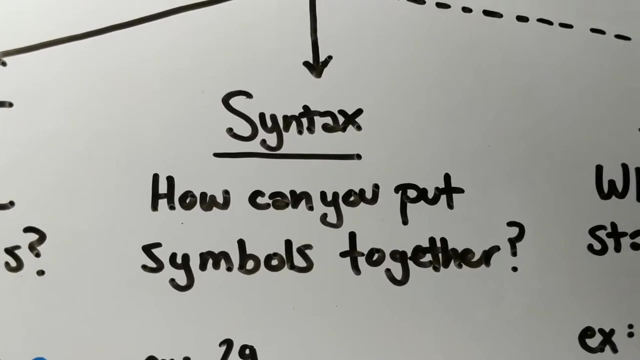 that's what an alphabet is. You have some set of basic symbols, Um yeah, Um. the next thing that every formal language has is a syntax, which basically is: how are you allowed to put those languages, those symbols together in order to form larger, um complexes of built out of those symbols? 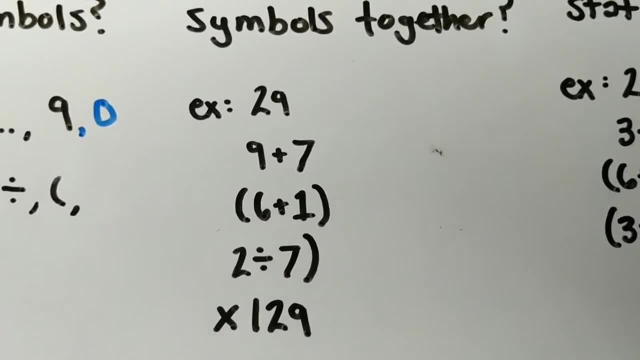 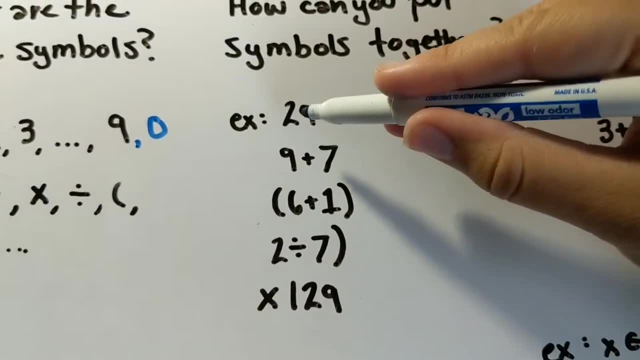 Um. so, for example, um, we're all pretty familiar with the language of basic mathematics, right? So we know that we are allowed to say um classic grammar Here you are allowed to share here in parentheses, and it has some meaning. 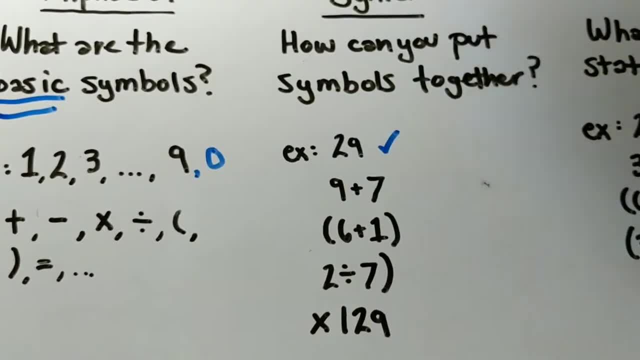 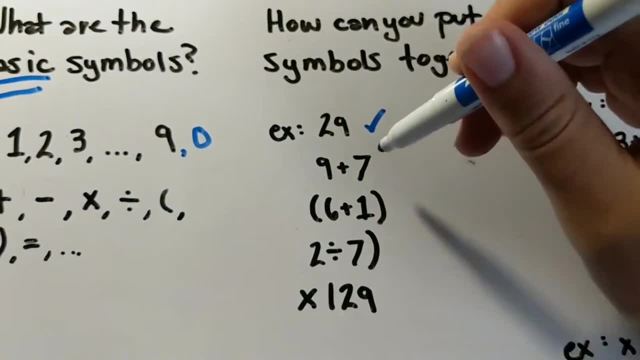 Um, remember this. there is a meaning in ideas, Right? um, two plus 9وت, and that has some meaning in basic mathematics, right, That 2 followed by a nine is allowed. You can have it stand alone and it can have some meaning, right. 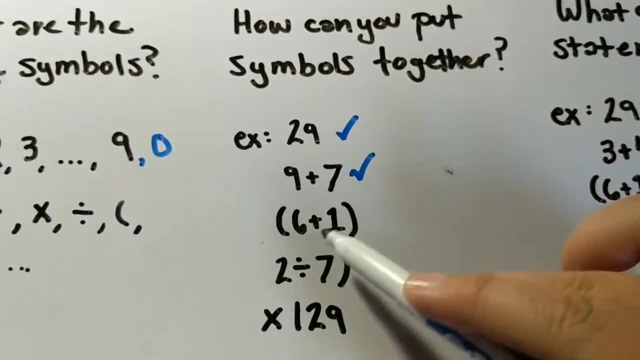 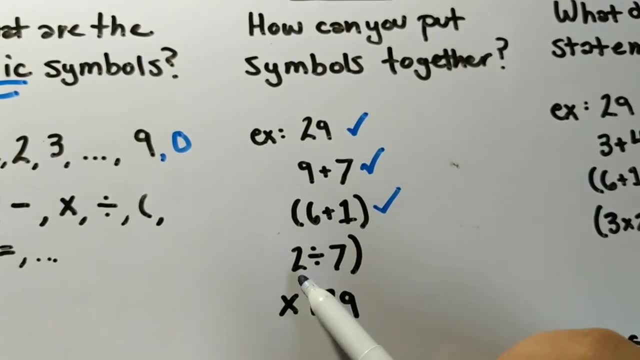 Similarly, 9 plus seven, um. that is allowed. you are allowed to combine symbols in that way. Six plus 1 in parentheses. you're allowed to combine symbols in that way. That's good. You are not allowed to use just one parentheses, right. 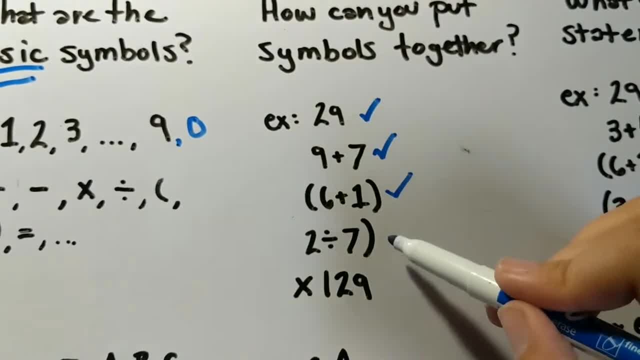 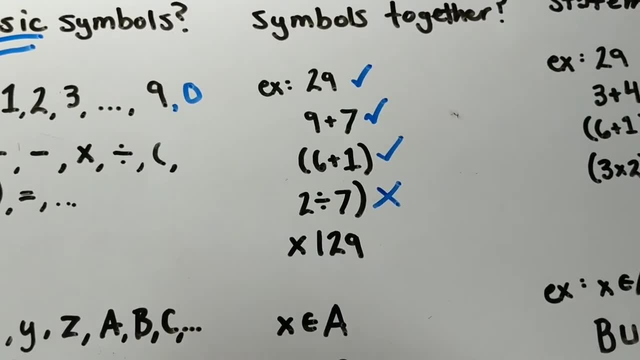 Um, Are you allowed to use just one parentheses in that way? Sorry, I'm sorry I can't say that, but by 7 close paren. that's not allowed right. so that is not allowed based on our syntax right. you are not allowed to say times 129 without having something. 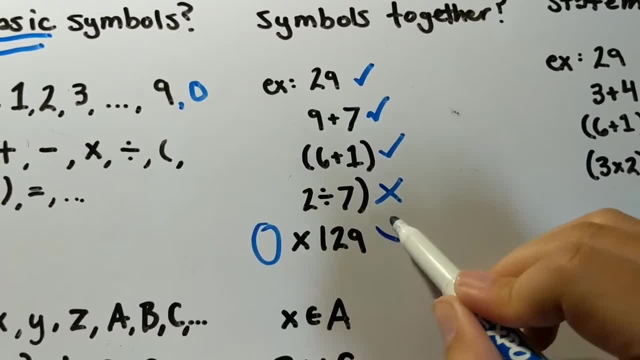 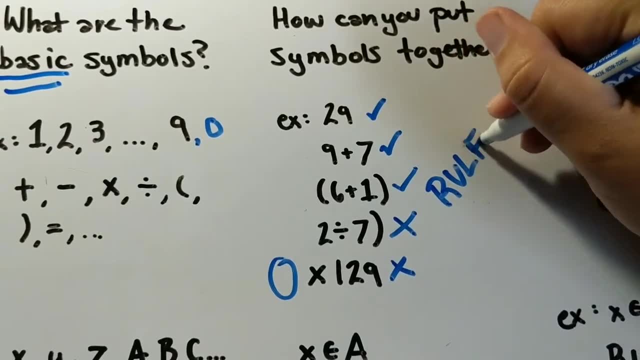 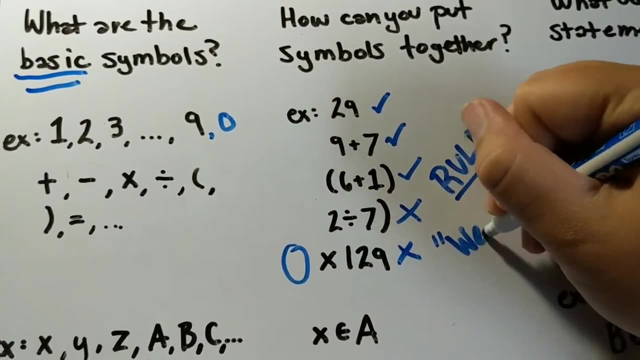 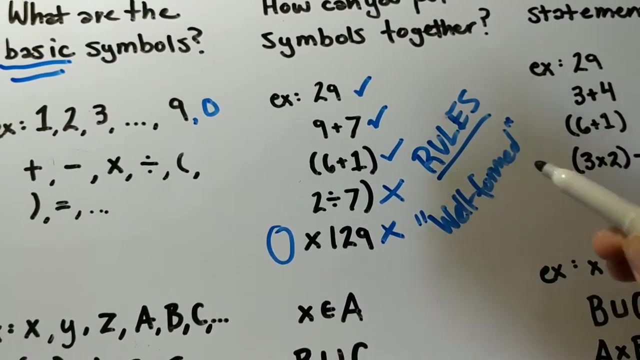 out here that is being multiplied by 129, so that is not allowed in our syntax. so the syntax is the rules that you're going to use to decide whether this is called a well-formed formula, right, so whether it's well formed, we'll go over this in the next video. so sorry that's a little scrawly, but we'll go over this. 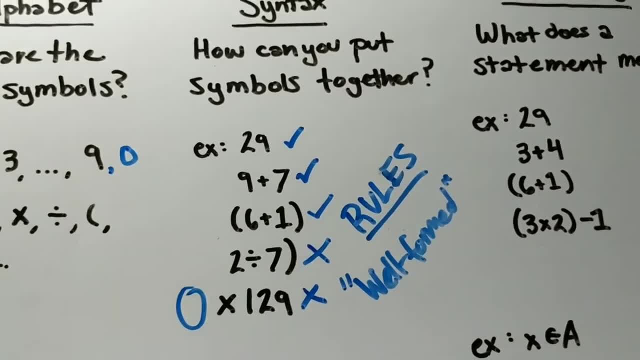 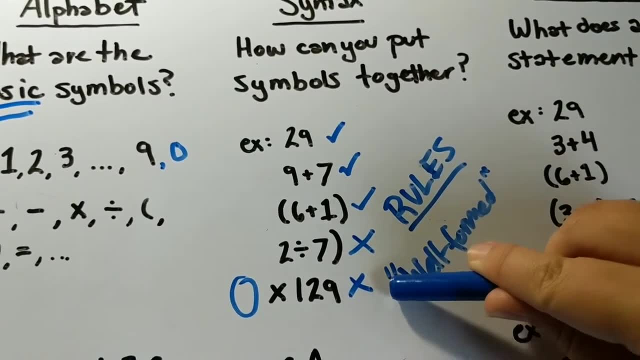 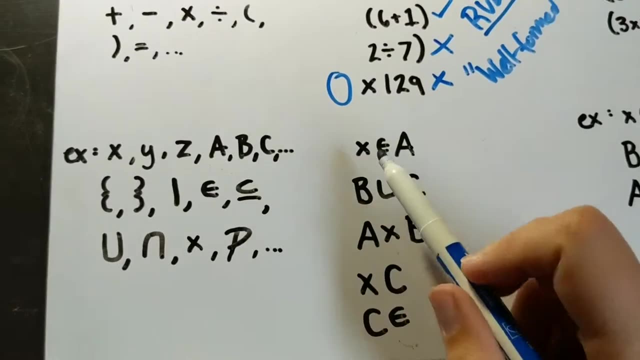 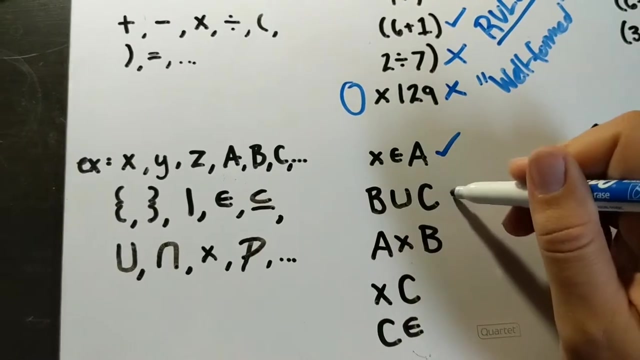 more when we start talking about the syntax of formal logic. right, so the syntax determines whether you are allowed to combine symbols in that way. your basic alphabet symbols, right? we can do this with the set theory as well, right, so, um, um. are you allowed to combine x, member a, that is fine. b, union c, that is fine a. 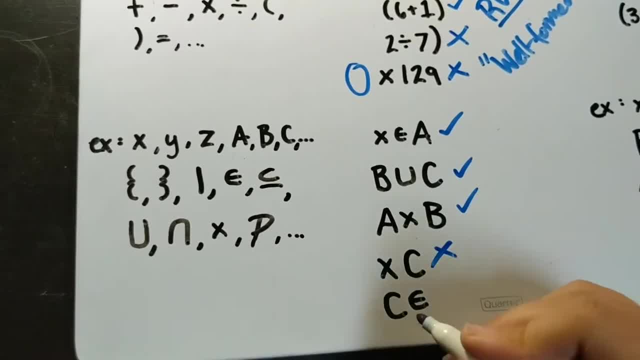 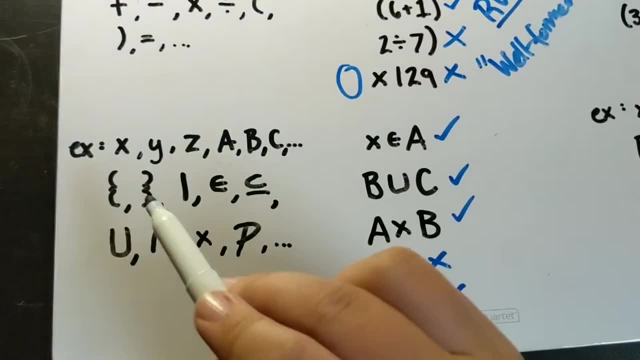 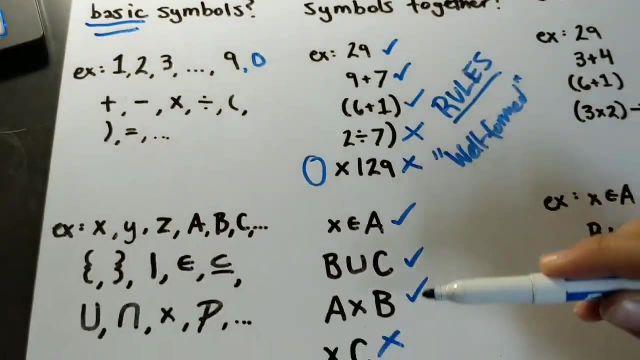 cross b, that is fine. cross x: not allowed. c- member of nothing is not allowed, because there are certain rules that determine how you are allowed to combine these symbols into larger complexes of symbols. right, and this has nothing to do with the meaning of them. right, you could probably determine the meaning of. 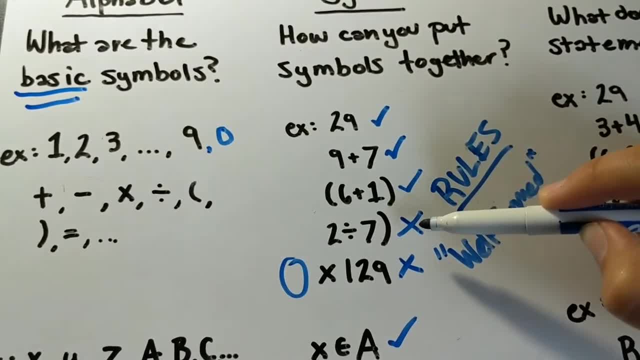 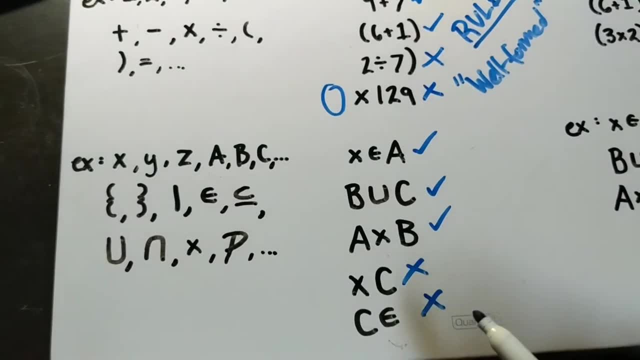 this, for example: right, two divided by seven, close paren. you would just be like, well, it's probably just two divided by seven, whatever that is, I don't know. but you know you can't always define a meaning, but you could probably figure out that meaning. but it's still not allowed. you're still not allowed to say: 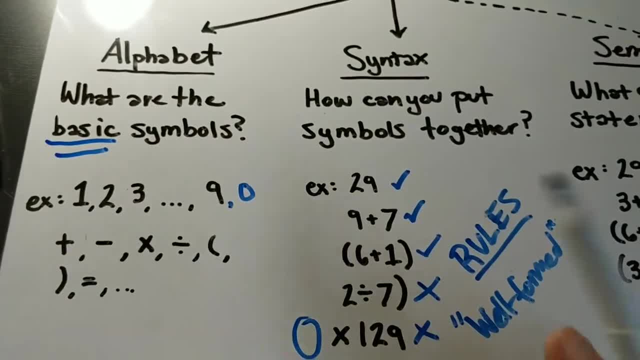 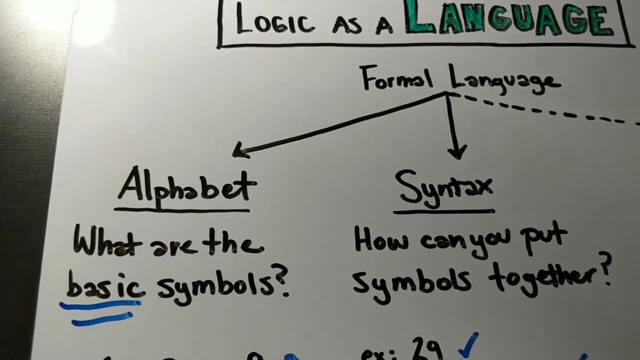 that right. so the syntax is a set of rules about how your symbols can be put together, so that is all that is required for a formal language. so, in theory, you could have a language that's just a series of meaningless symbols that are meaningless symbols where you never assign a meaning to them. it's just 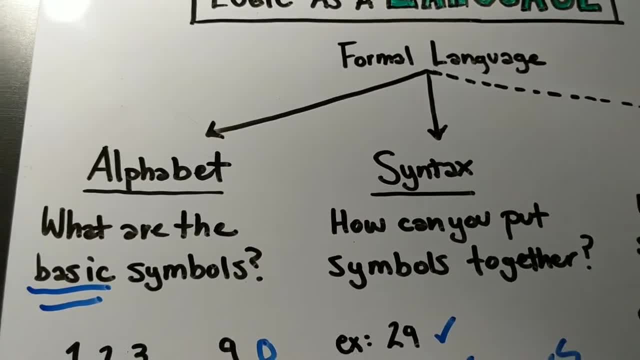 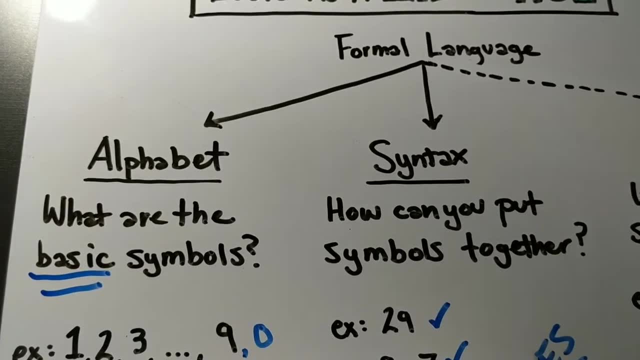 you're only allowed to combine them in certain ways, and we'll see a lot of those when we start talking about formal language theory. because those are good ones to play with to understand formal languages, because then you don't have to worry about the semantics coming in to interfere. all right so, but the final. 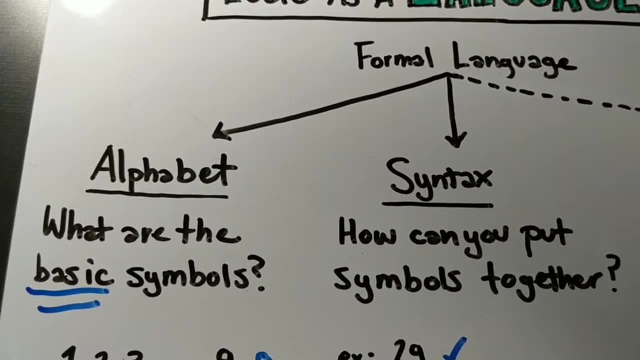 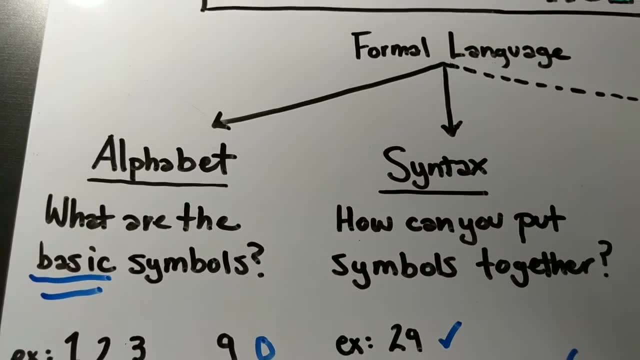 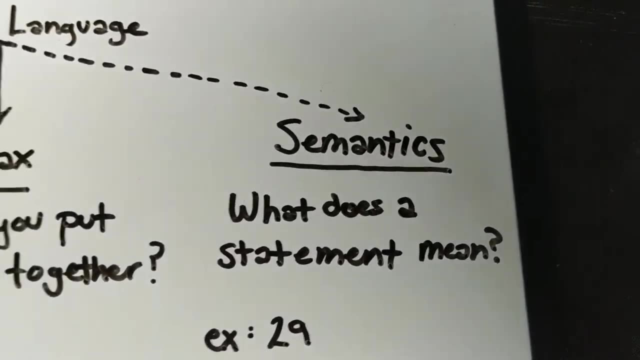 thing that many formal languages have, especially formalized versions of natural language, for example, or computer programming languages, which are formal languages or formal logic, as we will see- is that they have a semantics which allows you to take these combined sets of symbols and give them some sort of deeper meaning. 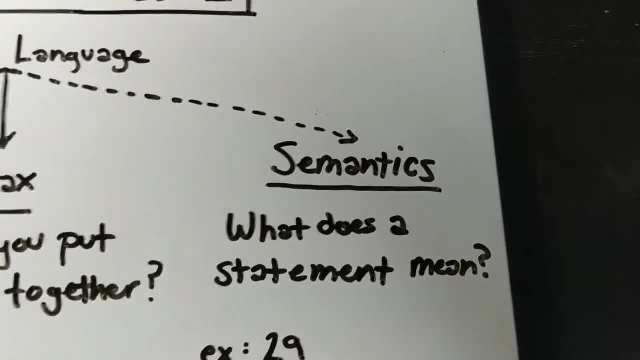 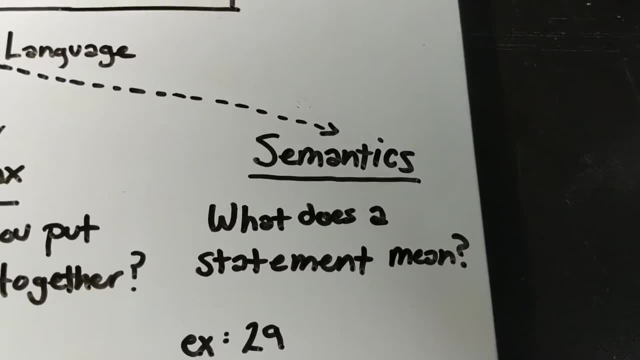 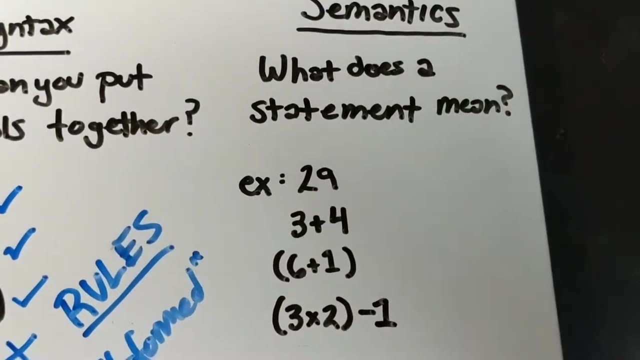 right, whatever you determine that deeper meaning to be is gonna be what your semantics is. so the semantics can either very much abstract a statement like this or it can just simplify it. so, for example, the statement 29: right, we have these two symbols next to each other. this doesn't. 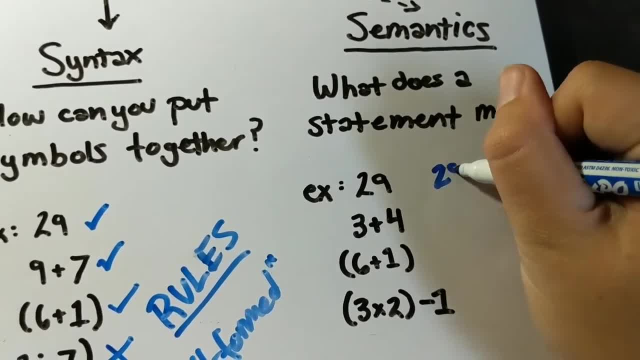 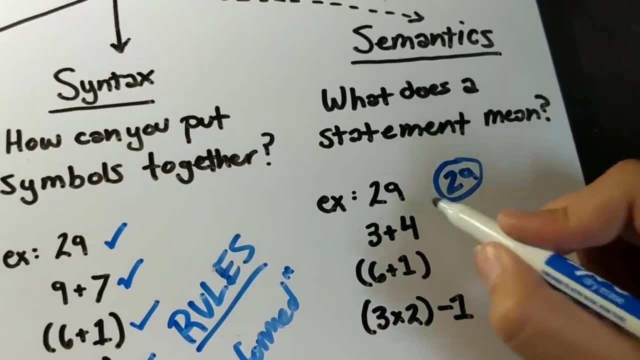 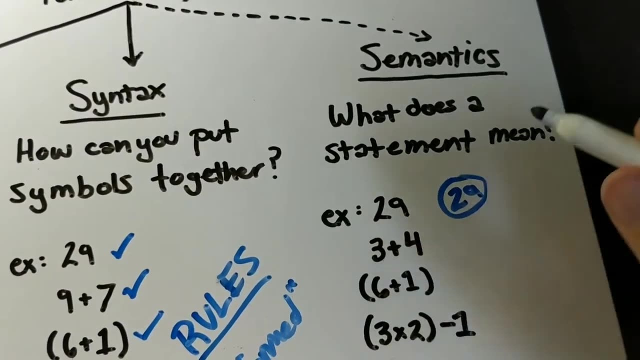 mean like two and nine. right, it means 29, which is a different meaning from two, followed, you know, from two and nine just occurring together. right, there's a. there is a separate thing out there in the world that is 29. that is, you know, way more than ten, right, three plus four. we can answer with another symbol as seven. 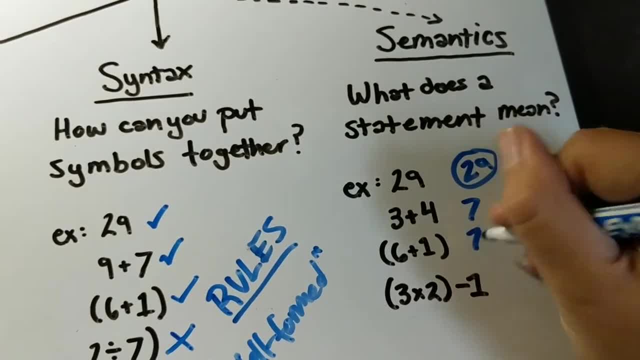 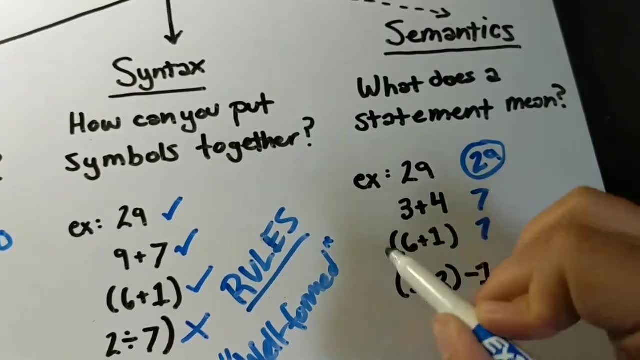 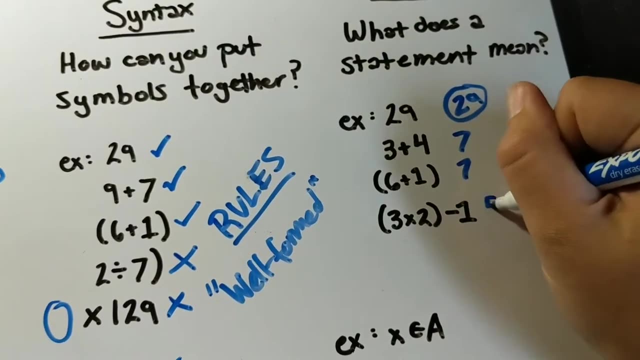 right. six plus one is in parentheses- is also seven. right, so this is assigning a semantics. there is a meaning that we can take out of this statement, which is well formed: right, three times two in parentheses, is six minus one is five. right, and that is the meaning that statement. right, so the semantics is: 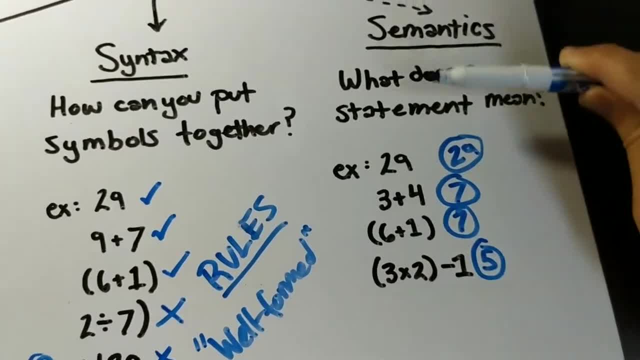 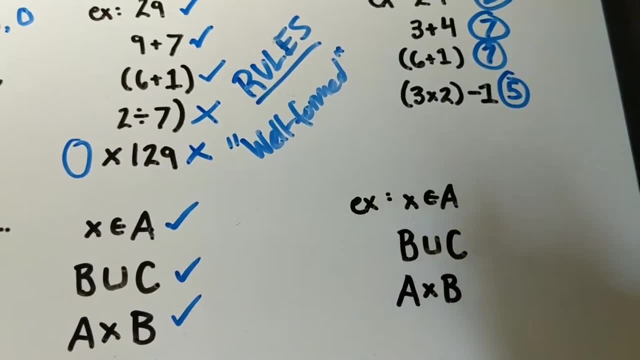 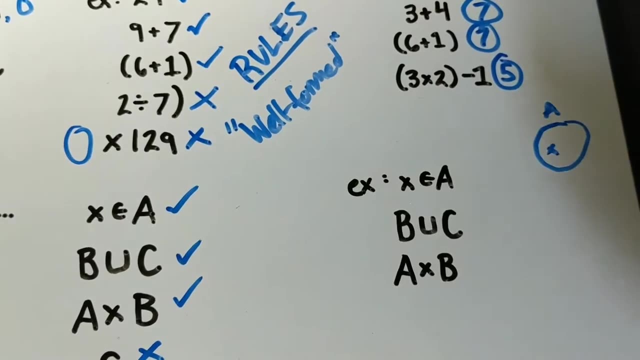 where you sort of solve a formula. right, we can think of that as solving a formula, right. this is a little more complicated when we start looking at set theory, right? so X is a member of a means something a little bit abstract. it means you have some set a and X is in it, right? we don't really have a good way to write. 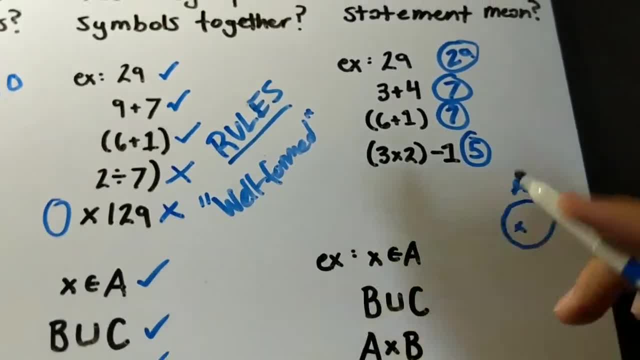 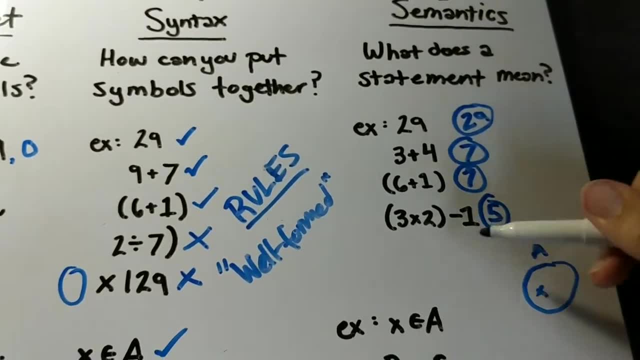 this other than X is a member of a right. it's not like this where we can just put down another number right. we can't give the semantics in terms of the same basic symbols that we're using- right B, union, C, we can sort of think of. 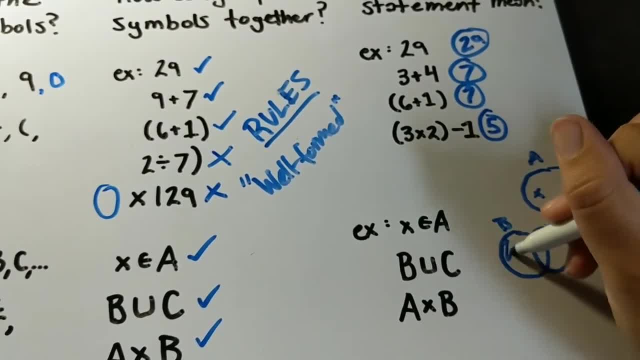 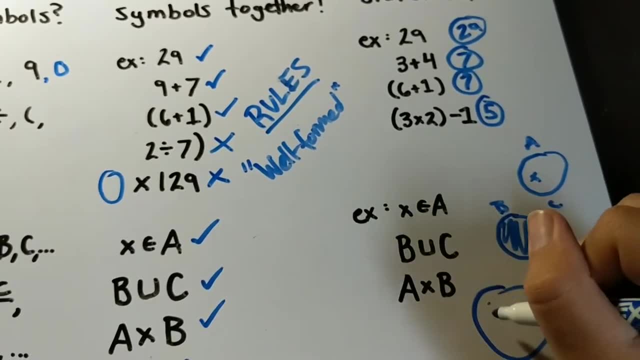 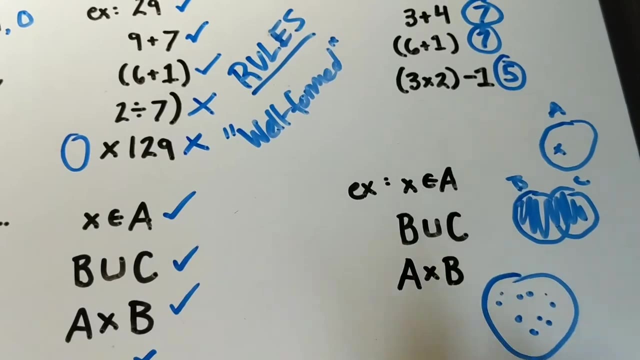 as two sets, B and C, and you know all of the stuff right: a cross B. similarly is going to be some other set which contains a bunch of things which are a cross B, right? so the semantics is how, once we're given a well-formed syntactic, 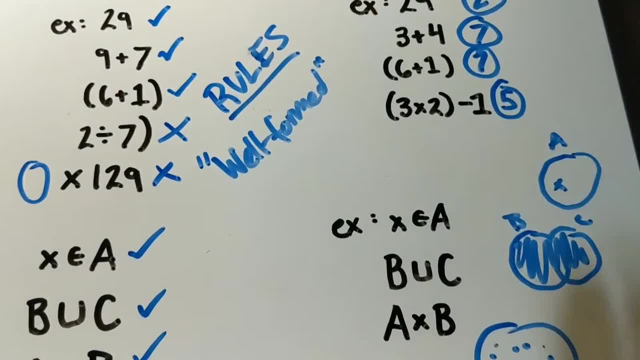 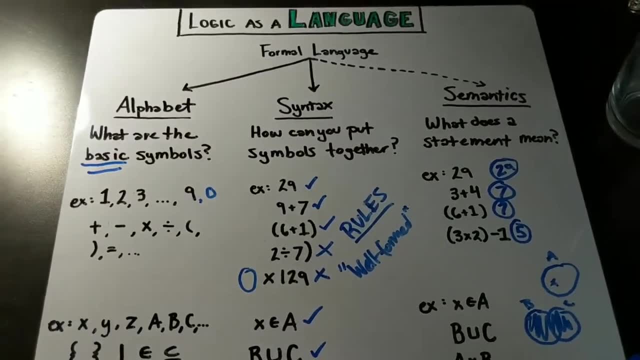 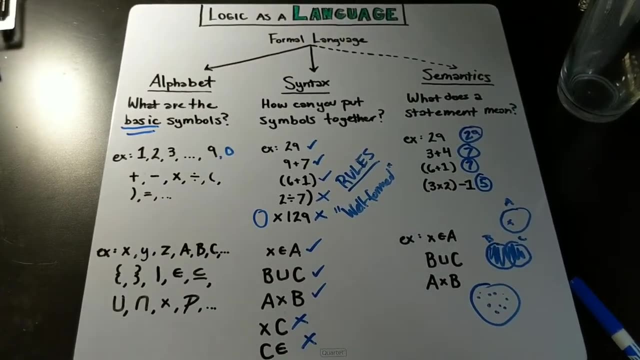 a syntactically well-formed piece of this formal language. what is it going to mean? so when we start applying this to formal logic, we are first going to learn the alphabet and the syntax, and then we'll start talking about the semantics and what it means. all right, so this has been your first little introduction to 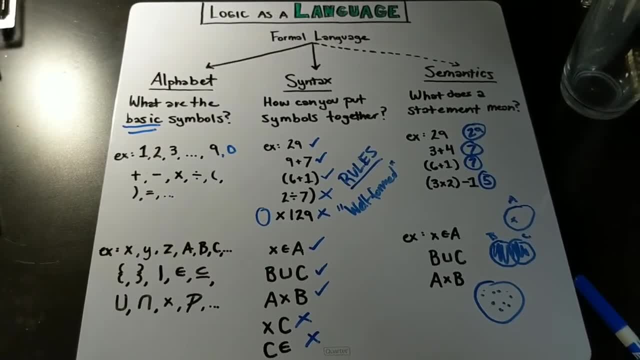 what it means to be a formal language and why formal logic would be perfect.